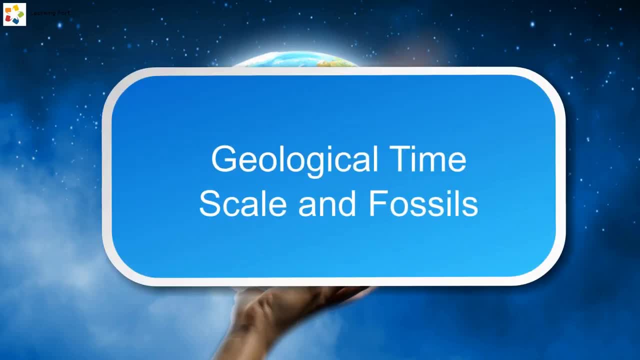 Earth is the third planet from the Sun. The Earth is estimated to be about 4.5 billion years old. Scientists used lunar samples and meteorites to determine the age of the Earth. 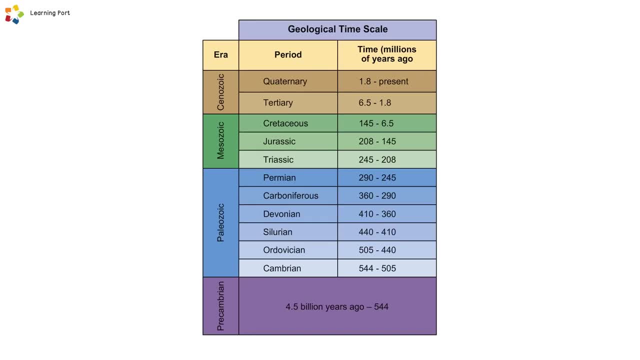 Scientists use the geological timescale to record various stages in Earth's history. Organisms define a long period of time as an era. Each era is divided into several periods. 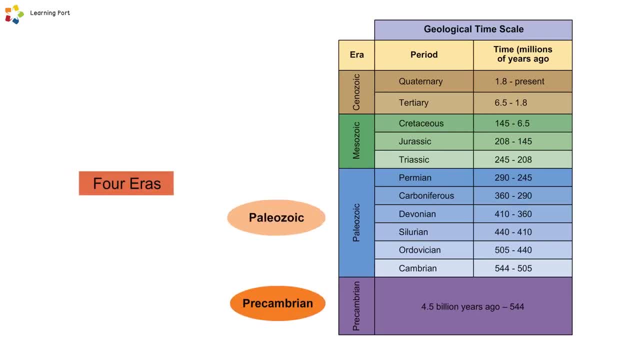 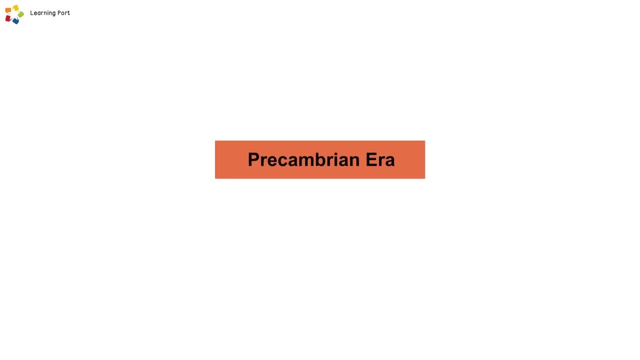 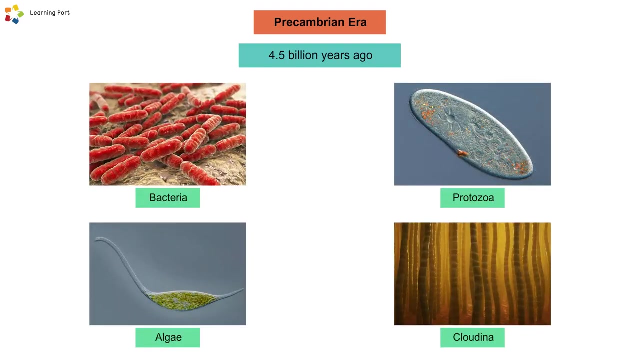 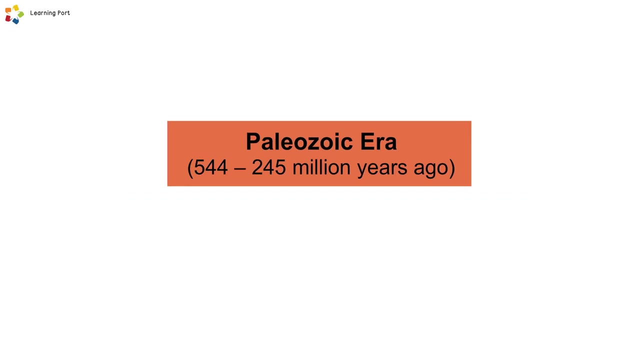 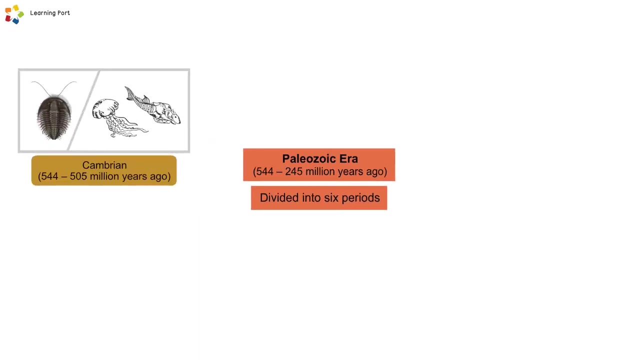 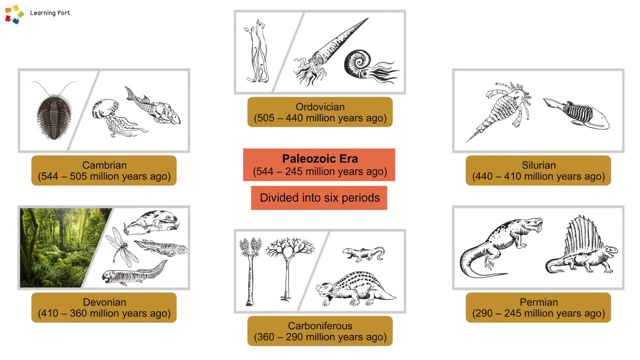 There are four eras, Precambrian, Paleozoic, Mesozoic, and Cenozoic. The Precambrian era began when Earth was first formed, 4.5 billion years ago. The earliest living organisms to evolve were simple organisms. The Paleozoic era lasted from 544 to 245 million years ago. It is divided into six periods. Cambrian, Ordovician, Silurian, Devonian, Carboniferous, and Permian. 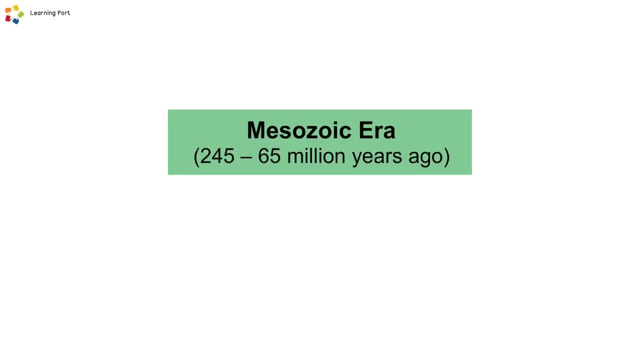 The Mesozoic era lasted from 544 to 245 million years ago. It is divided into six periods. Cambrian, Ordovician, Silurian, Terminatorian, Dad 현재ossi, longevanus, Pap ожидus, and Geomanceros gehört. 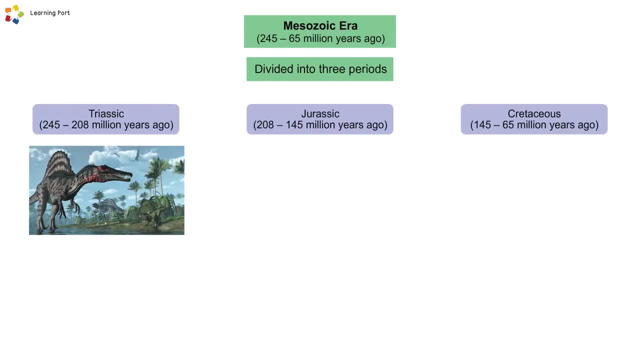 The first mammal and dinosaur evolved during the Triassic period. 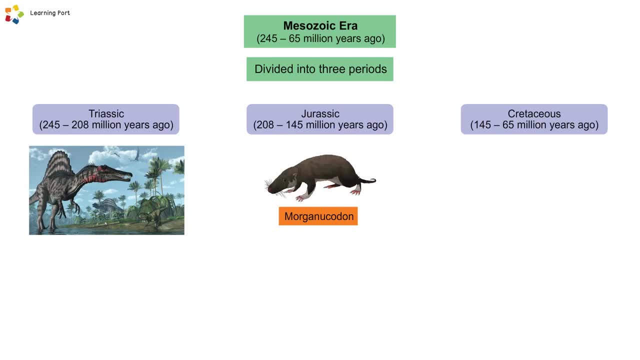 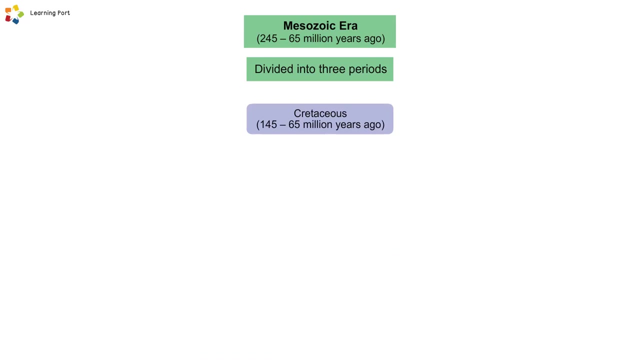 Morganugadon was one of the earliest mammals that lived during the Jurassic period. The first nonflowering plants such as conifer, palm-like cycad, and fern appeared during the Jurassic period. The Cretaceous period may have seen more dinosaurs than ever before. 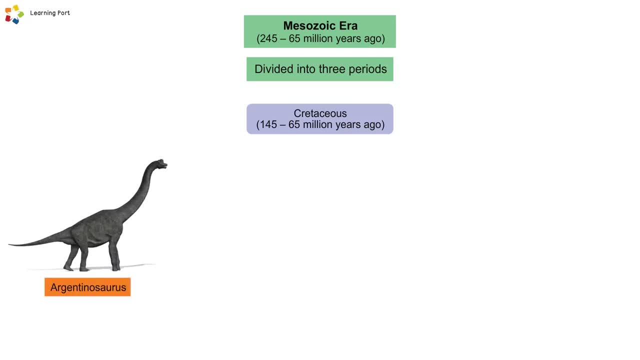 Dinosaurs that lived during this period were the Argentinosaurus, Tyrannosaurus, Triceratops, and Pteranodon. The Cenozoic era began 65 million years ago and continues into the present.